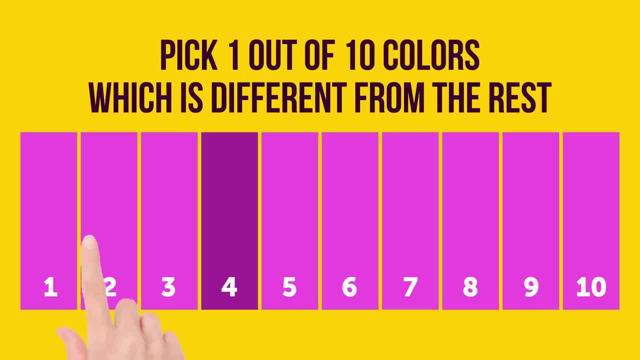 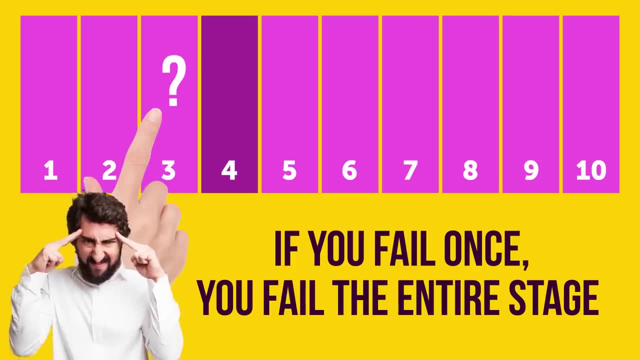 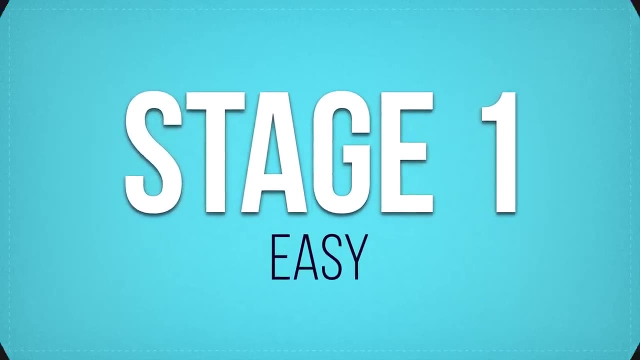 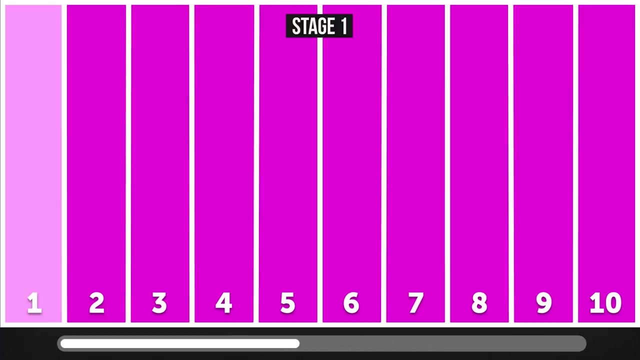 To pass each of the stages, you have to find that odd one out in each task. If you fail once, you fail the entire stage. Hey, no pressure, So sharpen up those eyeballs. Here's stage 1.. Okay, this one was easy. 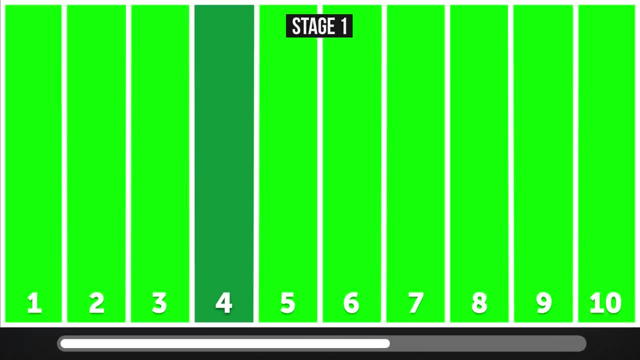 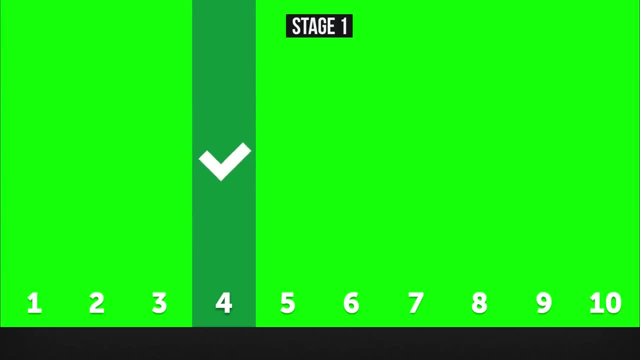 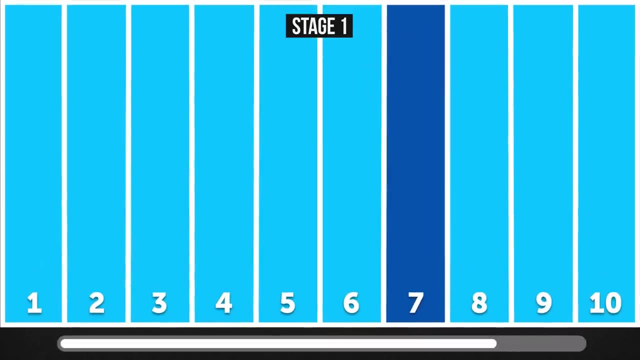 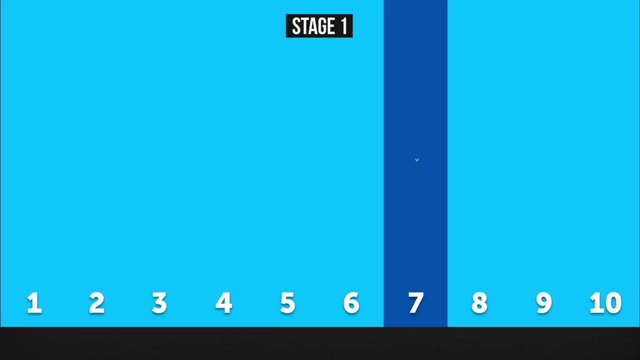 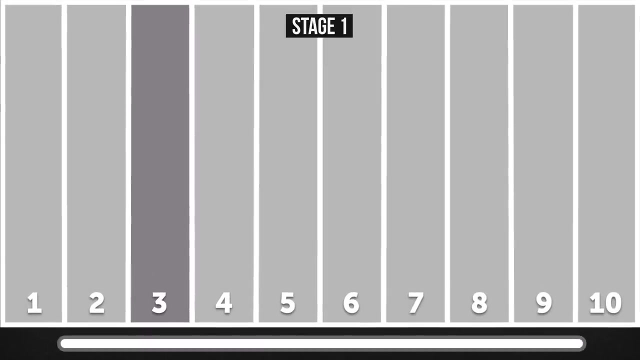 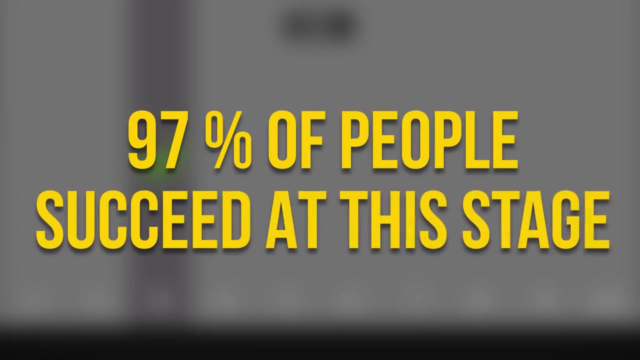 It's easier to find out what where yours are, Then identify a piece of material called the. You found a very strange creature. I hesitated a little. Done with stage 1?? It was just a warm-up. 97% of people succeed at this stage. 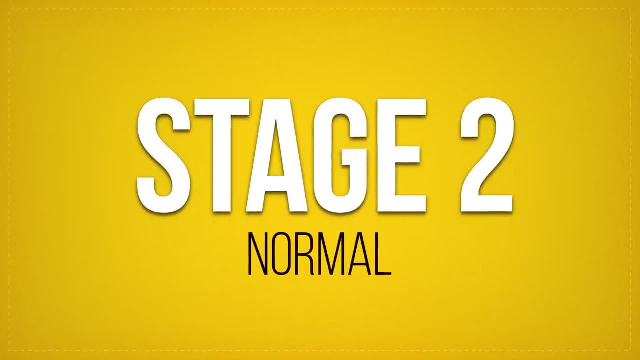 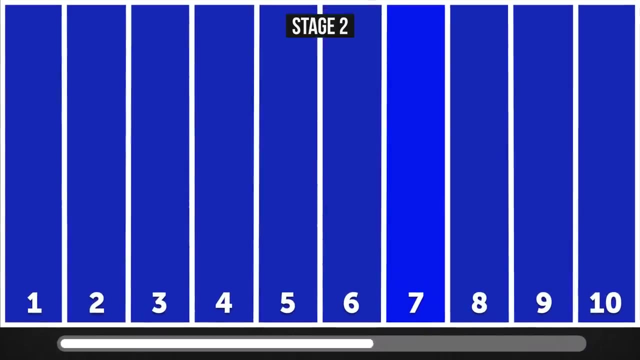 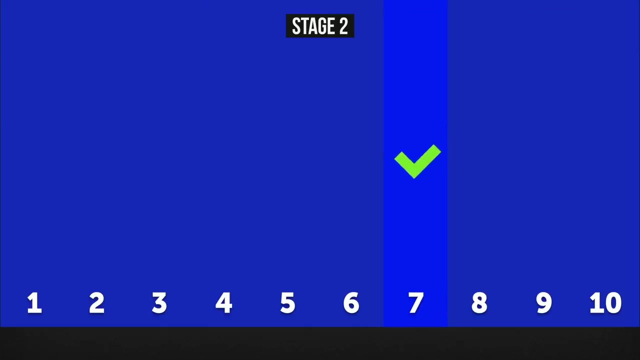 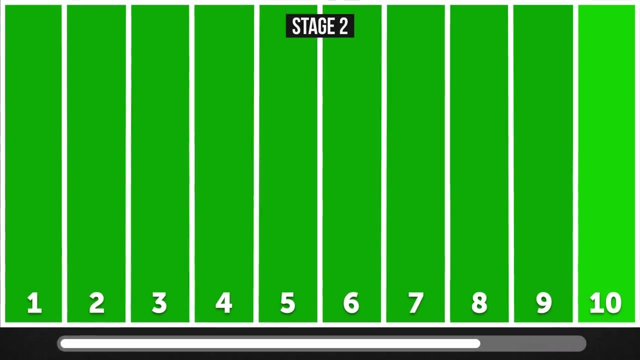 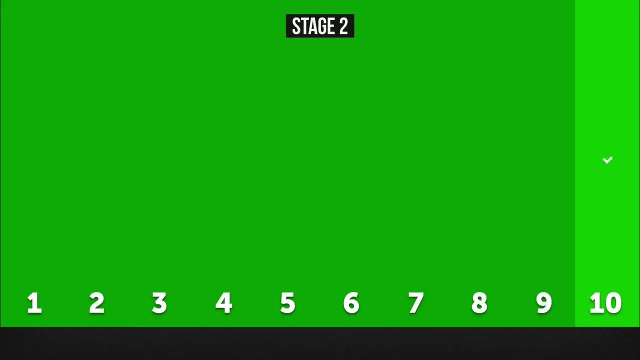 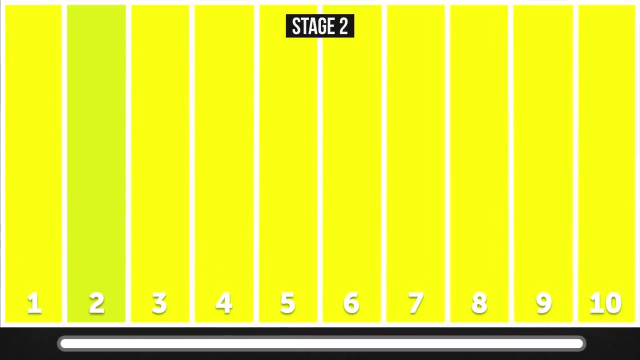 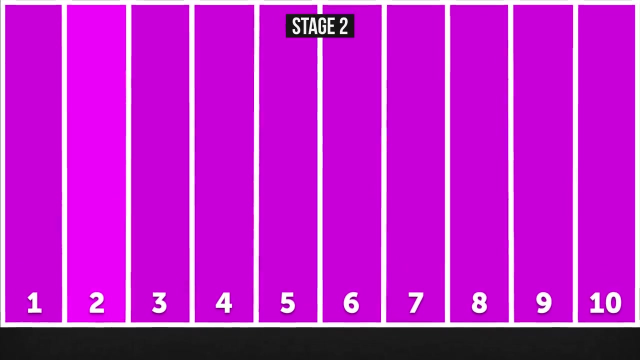 Stage 2.. Moving up on the difficulty scale, This one will require more attention. Hmm, let me take a look at this one. Yes, I knew it was number 10.. This one is tricky, Still winning at it. This one is tricky. 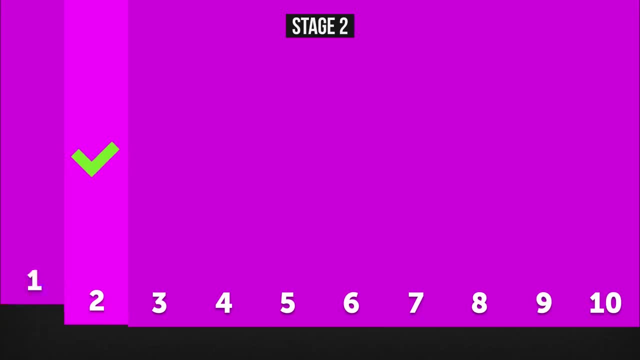 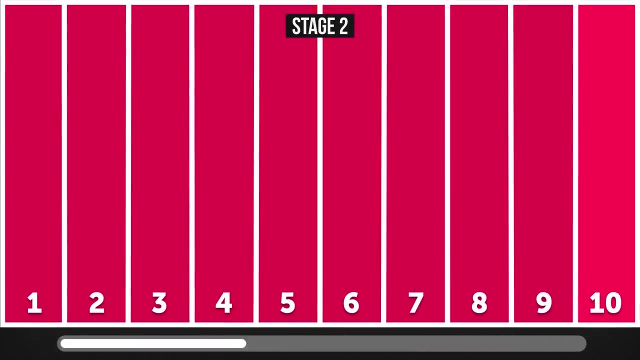 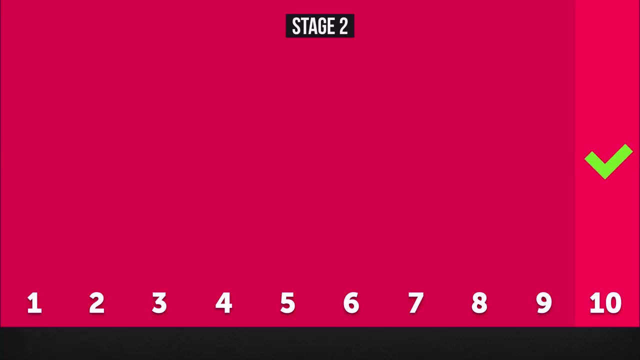 Level 3.. Was it not as easy? No, 実력ские 더 고이기. Stage 2 is over. Did you make it? Hit thumbs up if you did. In that case, you have a healthy. 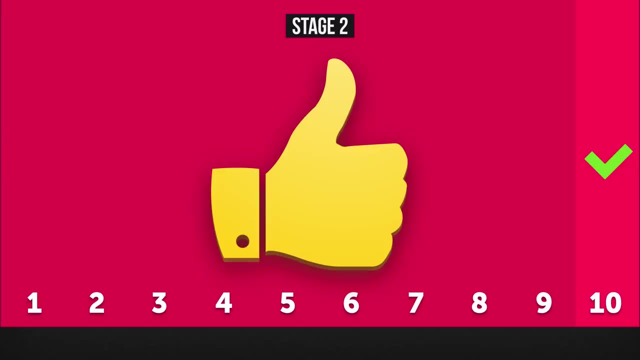 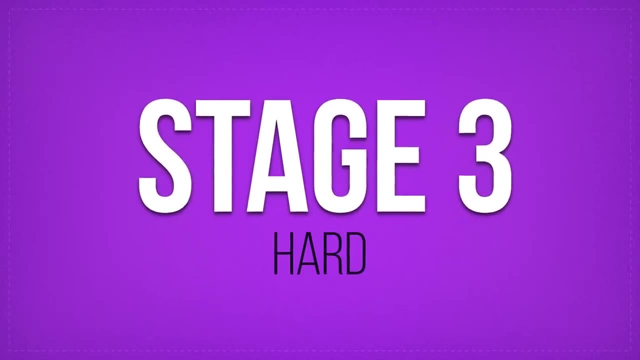 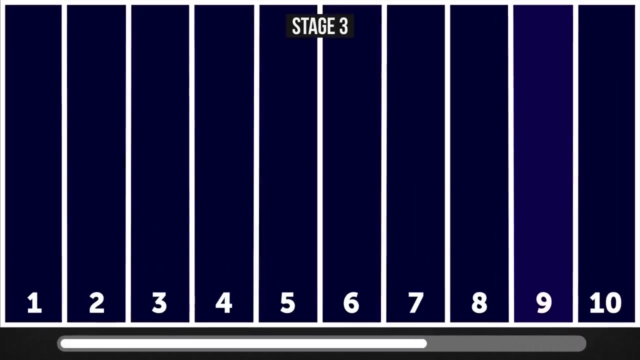 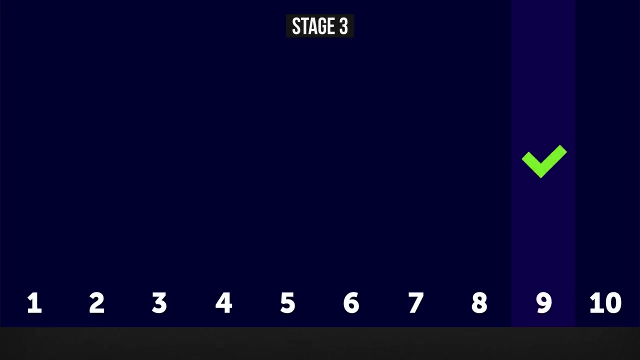 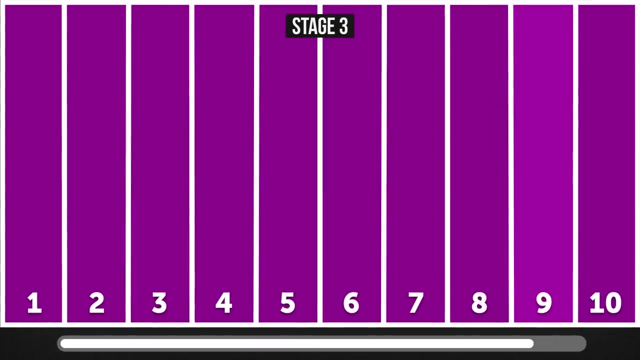 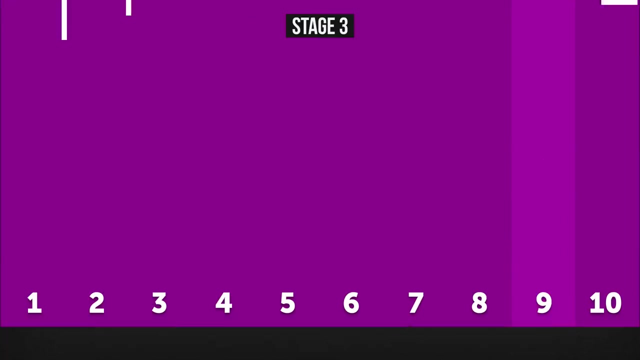 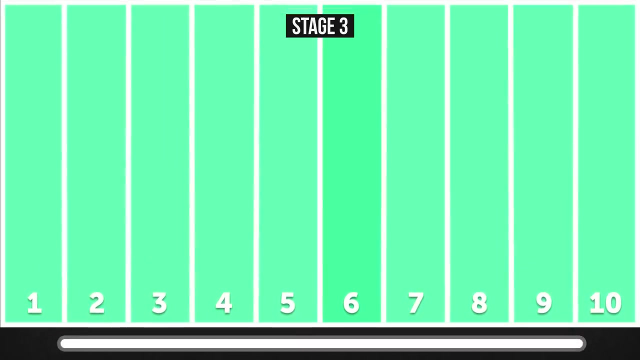 average eyesight, just like 55% of all test takers. The challenge is getting tougher and tougher. Get ready for stage 3!. Wow, that was very subtle. You're doing great. These 50 shades of turquoise are not really different, are they? 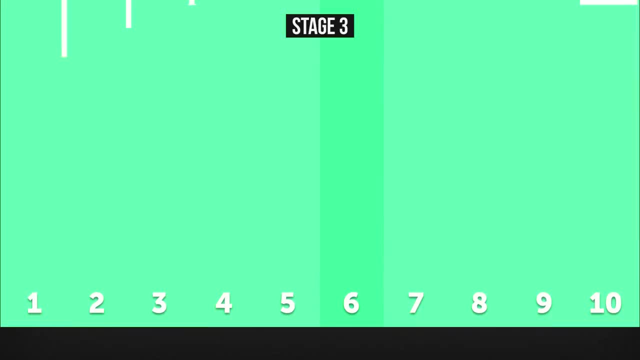 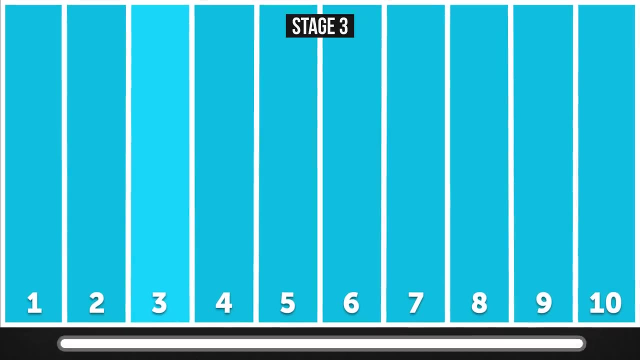 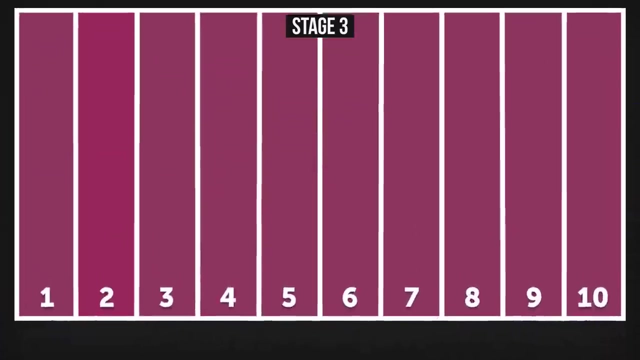 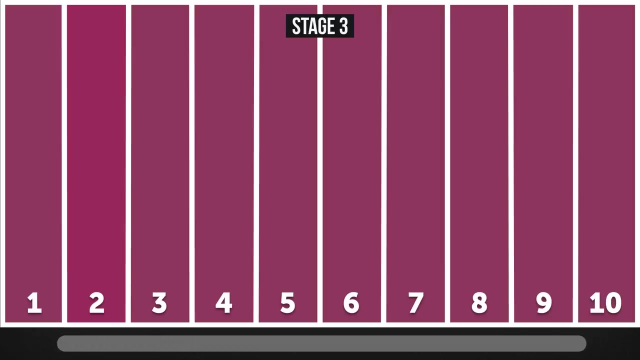 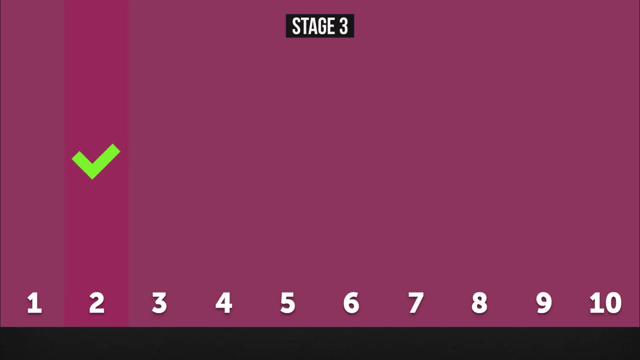 Oh, I see it now. Wow, You're doing great. You're doing great Done with stage 3! Congratulations to those who made it. You stand with the 30% of people who made it too. In case, this was the stage you failed. 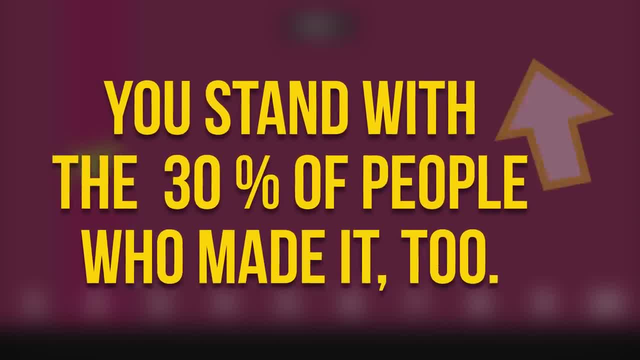 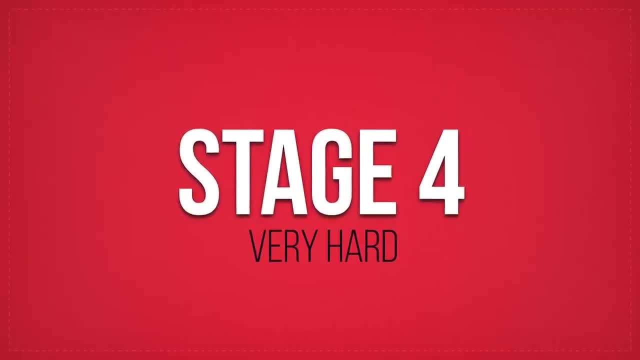 In case this was the stage you failed, don't be sad. you can improve your eyesight, and this video will tell you how to do it. and this video will tell you how to do it. And now it's time for stage 4!. 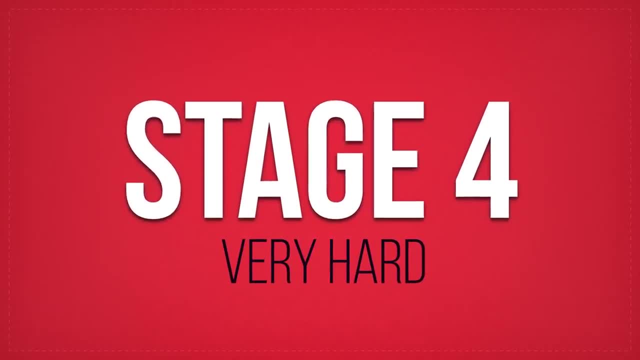 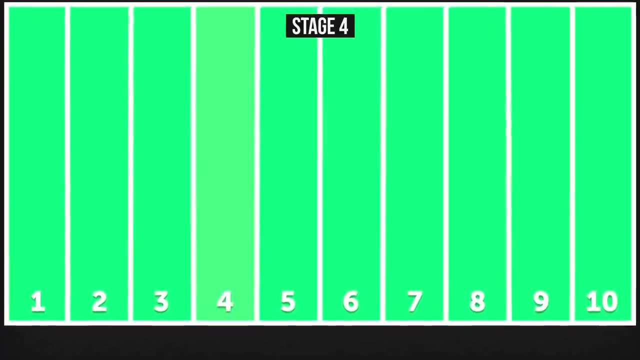 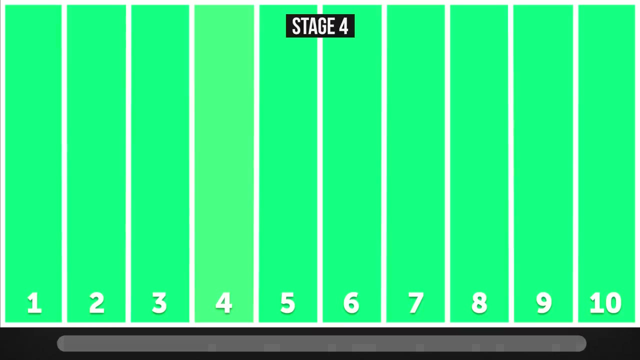 Caution: it might change your life because you can discover some super powers in yourself. Ready set go, Ready set go, Ready set go. Are you kidding me? These are identical. These are identical. Oh, who could have thought this was the odd one out. 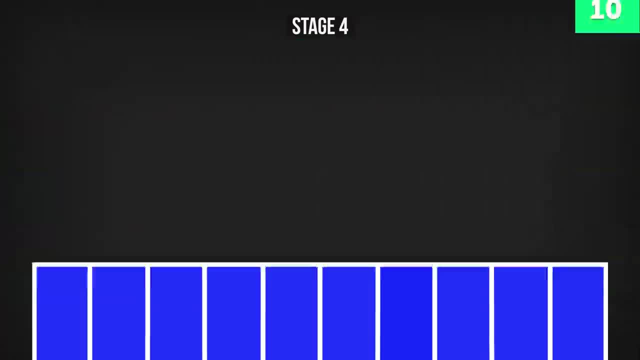 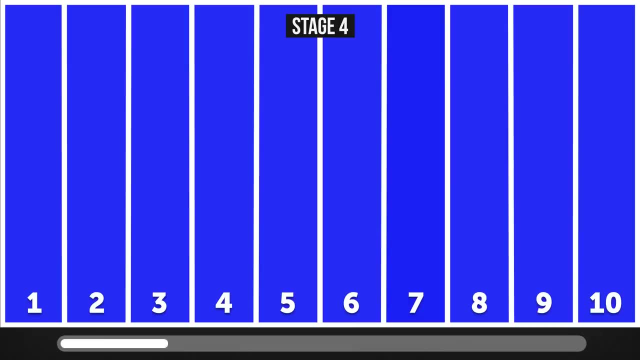 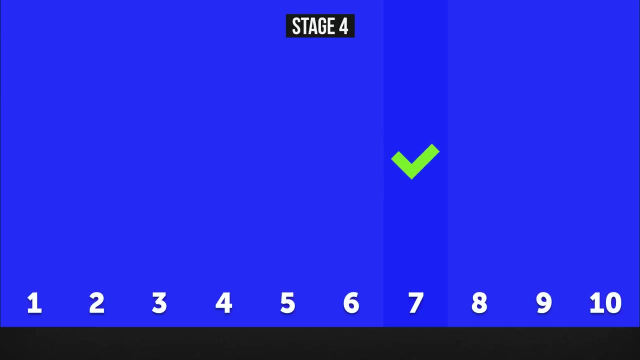 These are identical. These are identical. Let me clean my screen. Maybe it'll help me solve this one. No way, I thought it would be number 4.. I thought it would be number 4.. No, My device foiled.